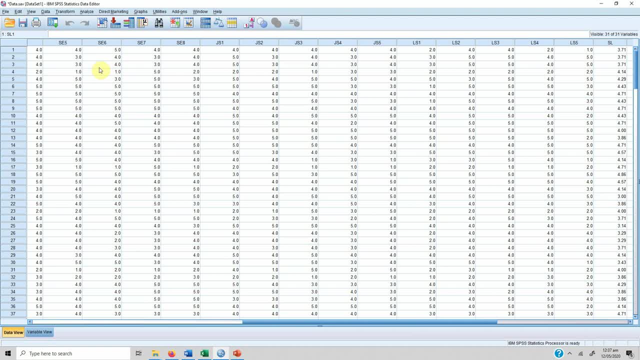 whether the correlation was same between the two groups or whether it was different. or if it was different, was it significantly different? Now, in order to do this, the first step is that we have to do is we have to split the file. We want to compare based on gender, so we select gender and we 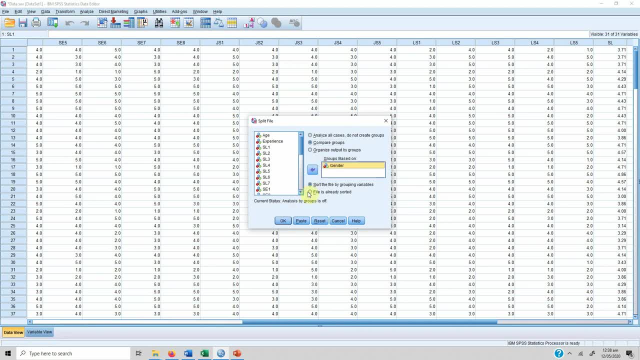 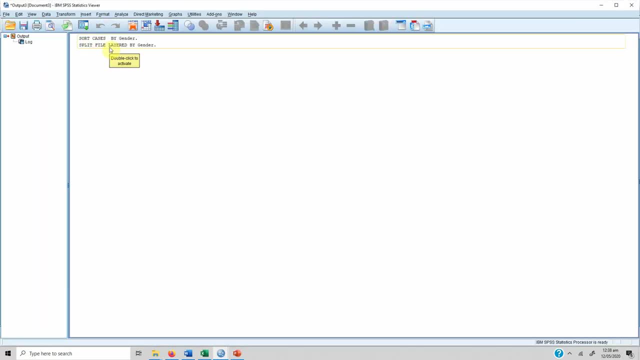 want to compare the groups. so we press this arrow. We don't need to do anything else, we just press OK. Now, split by gender. Now, in order to run the analysis, you go to analyze, you go to correlate and bivariate. Now we are all interested in servant leadership and self-efficacy. We want 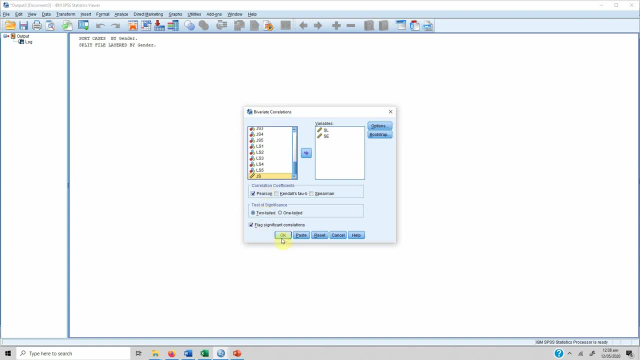 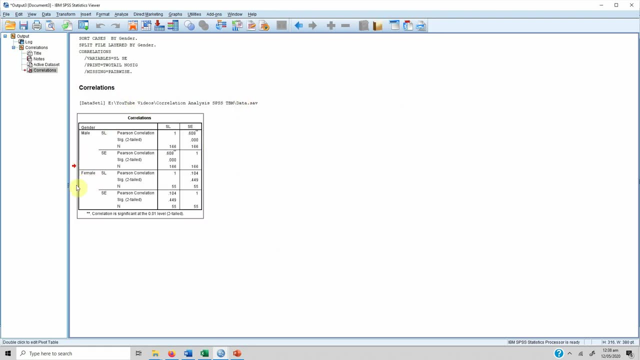 Pearson correlation. let it be two-tailed flag in significant flag, a significant correlation, and we press OK. Now if we see, here we've got correlation of SL with SE in male respondents and then we've got correlation of SL with SE in female respondents. Now if you look here, 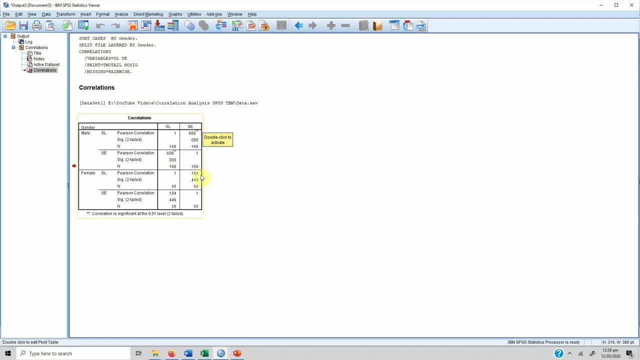 the correlation was significant in male respondents, but in female respondents it was insignificant. It was moderately positive in male, but it was very weak and insignificant in female. Now we know that there is a significant difference now between the correlation in male and females, but we want to do it. 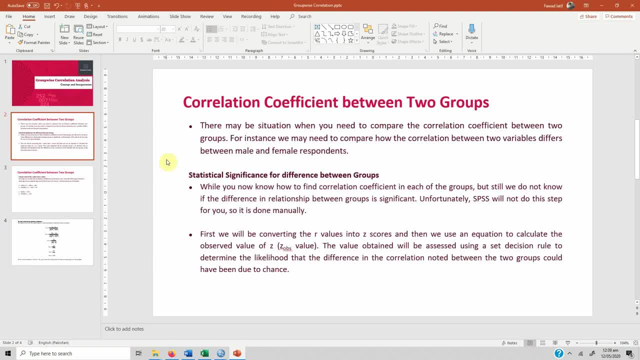 statistically. Now, in order to do this, let's go back While. you now know how to find correlation coefficient in each of the groups, but still we do not know if the difference in the relationship between these groups is significant. Now, unfortunately, SPSS will not. 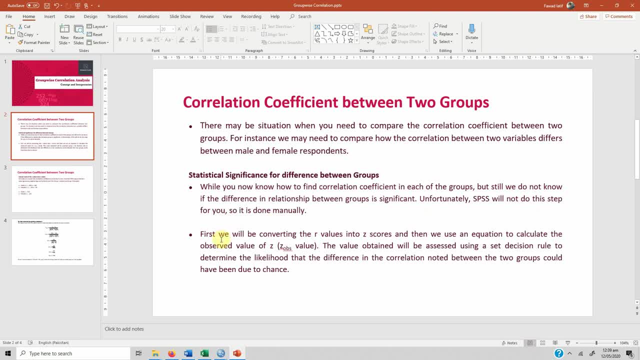 do this step for us, so we have to do it manually. Now, in order to do this, first we have to convert the R value, that is the correlation coefficient, into Z score, and then we use an equation to calculate the observed value of Z or Z score, that is, Z OBS value. 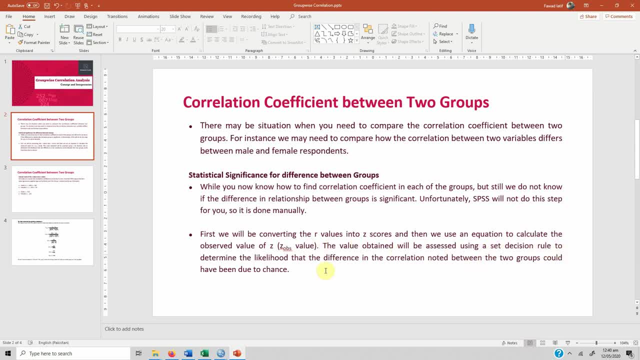 The value obtained will be assessed using a set decision rule to determine the likelihood that the difference in the correlation noted between the two groups could have been due to a chance or, in simple terms, whether or not the difference is significant or not. Now, in order to do this, the first step is we need the correlation. 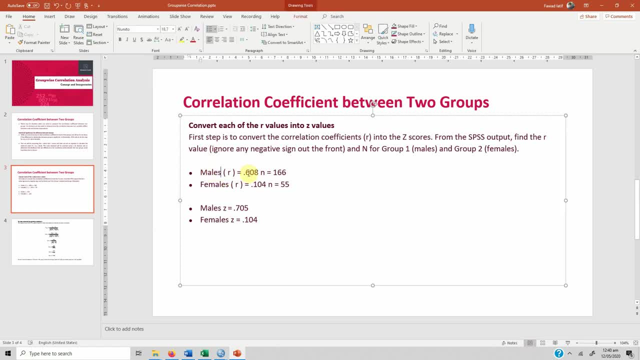 Now what I have done is I've already put in the values. the R for males was 608, while the N value was 166.. The R for females was 104, while the N value was 55. that is the sample size in each group. Now how do you convert this R score into Z score? It's very 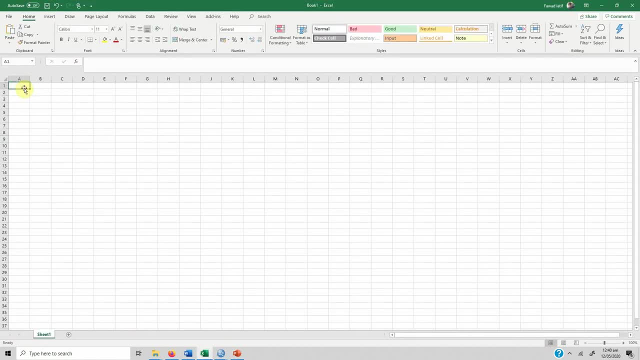 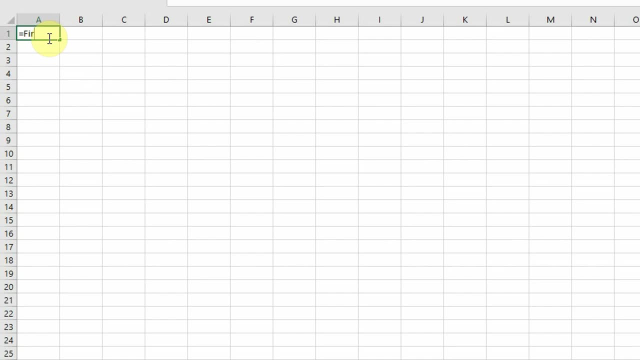 easy. we are going to use Fisher R to Z transformation in excel. So just simply press is equal to type Fisher and select the top value. And here you mentioned the value. so the correlation for males was 0.608. close the parenthetical bracket, press enter and now the value is: or the Z score value is 0.705. 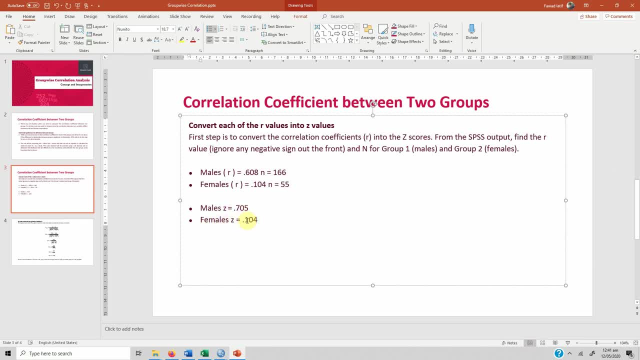 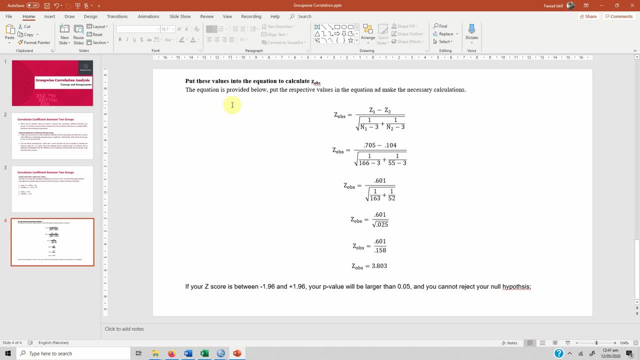 Here it is 0.705.. Now do the same for females as well. So, once you have these two values, what you are going to do is you are going to put it in this formula. The equation is provided below, put the respective values in the equation and make the necessary calculation. 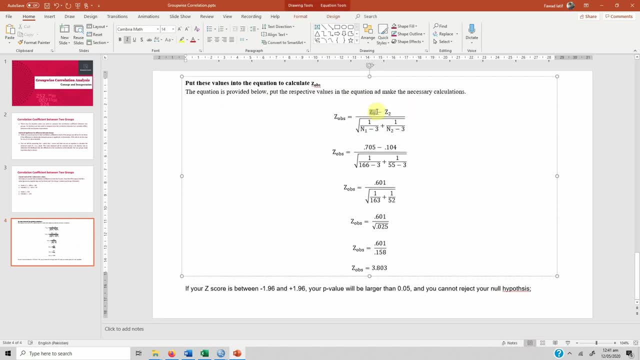 So Z observed score is actually Z1-Z2. so group 1-group 2, the N score for, or the number of respondents for group 1 and the number of respondents for group 2.. So what I have done is I have already added these values. So 166 is the N for group 1, male and 55 for. 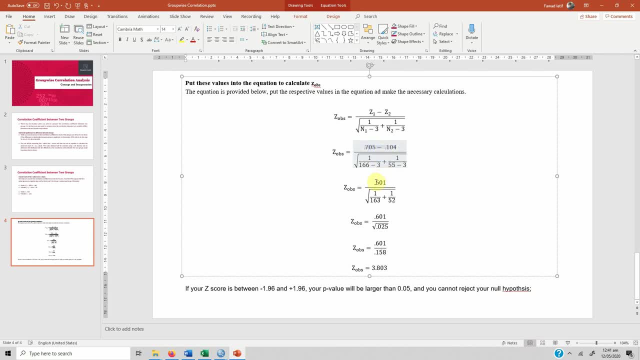 group 2.. Now you subtract, you get 0.601.. 163,, 164,, 165.. 552.. Divide these values and then add them. Take the square root of 0.025.. You get 0.15.. Divide.